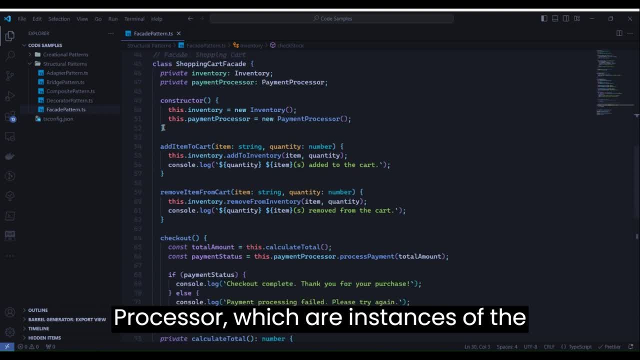 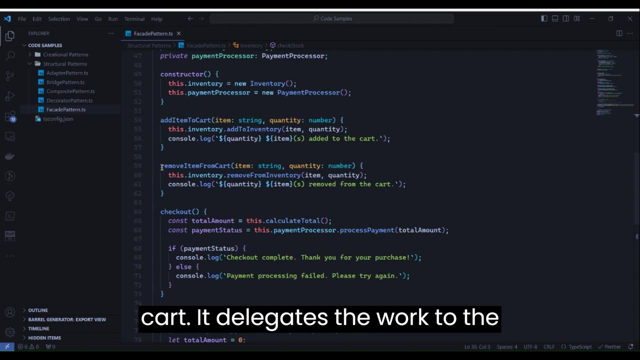 private properties, inventory and payment processor, which are instances of the inventory and payment processor classes respectively. The constructor initializes these subsystems. The add item to cart method simplifies the process of adding items to the shopping cart. It delidates the work to the inventory subsystem and logs a message indicating that items have 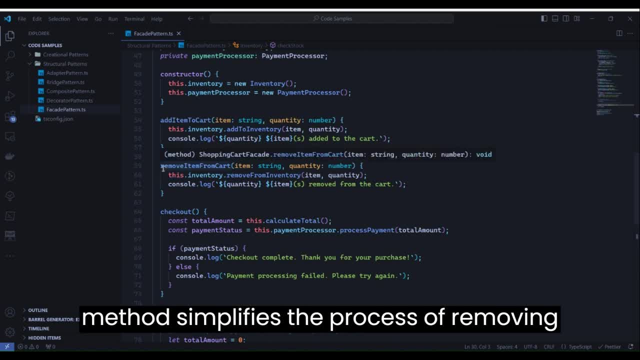 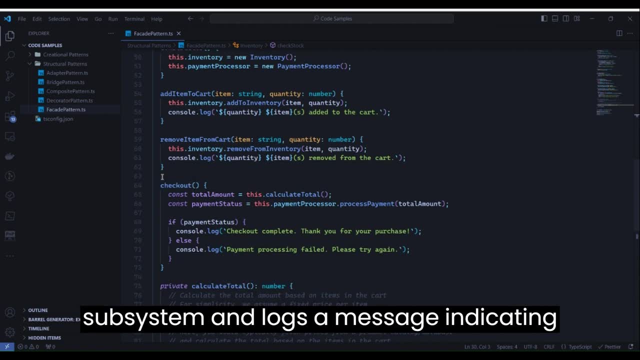 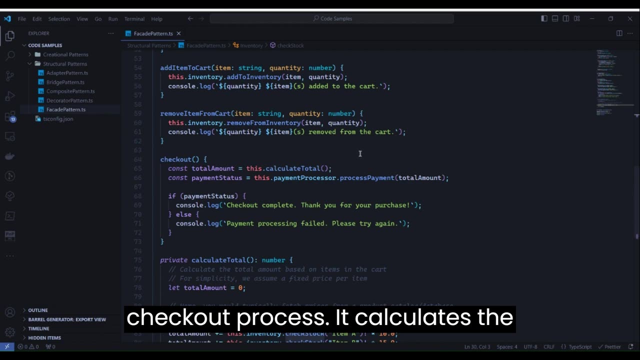 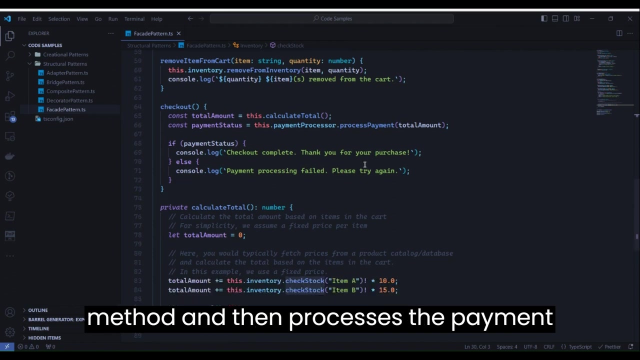 been added to the cart. The remove item from cart method simplifies the process of removing items from the shopping cart. The checkout method handles the checkout process. It calculates the total amount based on the items in the cart delegating to the calculate total method and then processes the payment using the. 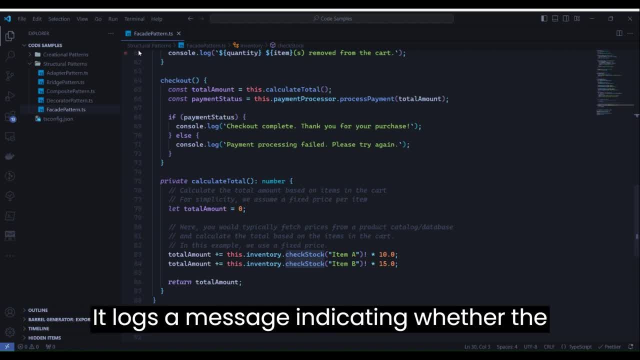 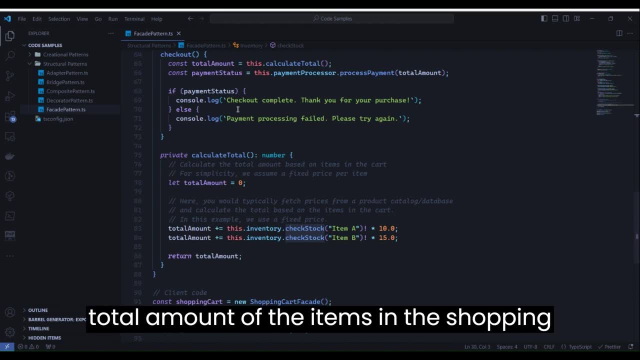 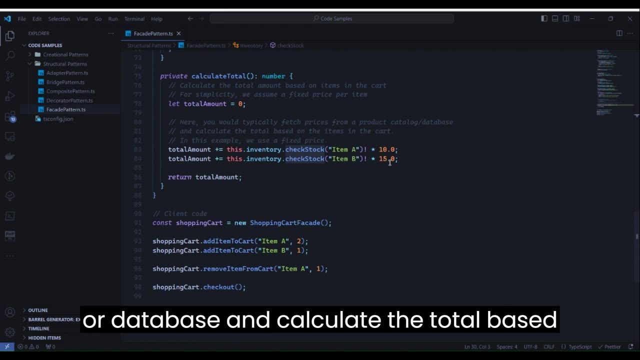 payment processor subsystem, It logs a message indicating whether the payment was successful or not. The calculate total method calculates the total amount of the items in the shopping cart. In a real-world scenario, you would fetch prices from a product catalog or database and calculate the total based on the items in the cart. In this example, it uses fixed prices for. 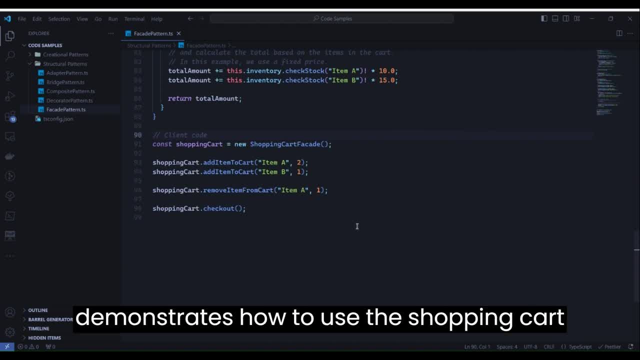 simplicity. The client code demonstrates how to use the shopping cart facade. It creates an instance of the shopping cart facade and then adds items to the cart, removes items and finally checks out The facade. simplifies these actions for the client, hiding the complexities of inventory. 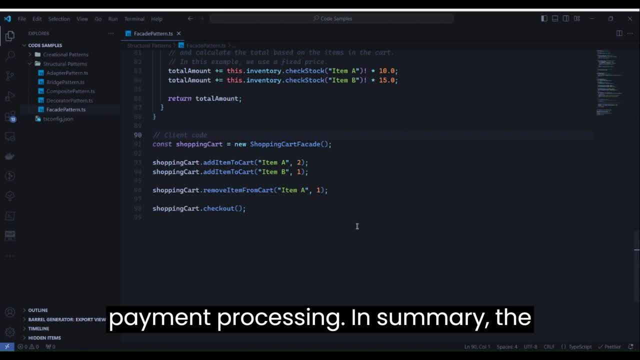 management and payment processing. The client code demonstrates how to use the shopping cart facade and payment processing. In summary, the facade design pattern simplifies the interaction between a client and a complex subsystem by providing a unified and easy-to-use interface. It abstracts: 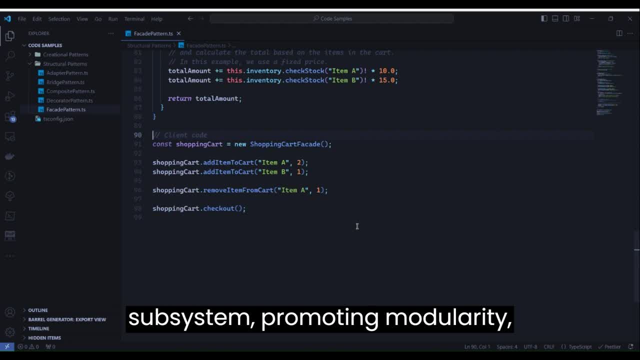 away the intricacies of the subsystem, promoting modularity, maintainability and ease of use in software systems. In this specific example, the facade pattern simplifies the management of an online shopping cart by encapsulating inventory management and payment processing, making it more. accessible to clients. In this example, the facade design pattern simplifies the interaction between a client and a complex subsystem by adding items to the cart. In this example, the facade design pattern simplifies the interaction between a client and a complex subsystem by adding items to the cart. In this example, the facade design pattern simplifies the interaction between a client and a complex subsystem by making it more accessible to clients. In this example, the facade design pattern simplifies the interaction between a client and a complex subsystem by adding items to the cart. In this example, the facade design. pattern simplifies the interaction between a client and a complex subsystem by adding items to the cart.